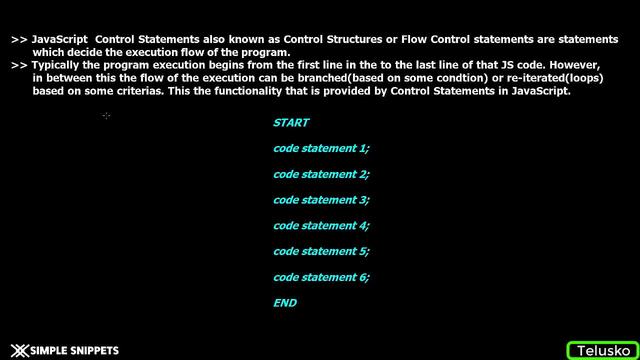 statements. So these control statements basically govern the execution flow of the program. So what do I mean by this? So, as you can see on the screen in the blue code, typically this is what happens. Let's say, we have the JavaScript code inside our script tag. Okay, 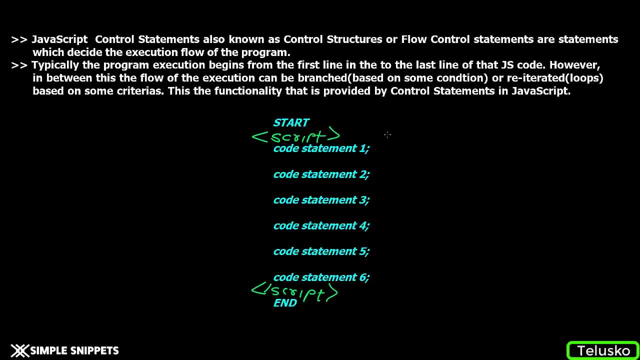 So this is our script tag. What happens is the execution starts from line number one, that is, code statement one, and then it moves on to the line number two, then line number three, and so on and so forth. So this is how the basic execution flow goes. However, in 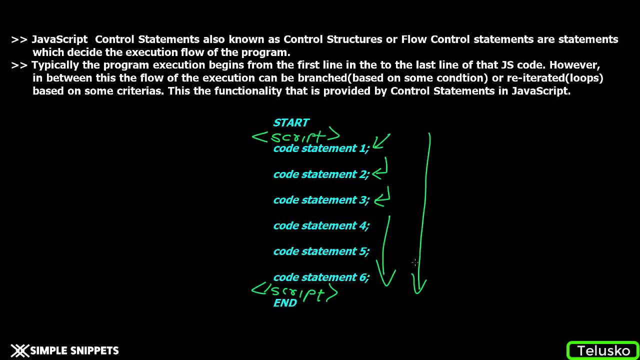 real time or in real world scenarios, this entire flow is not as simple as in this case. Okay, It is not going to be like a linear way in which the code is going to flow in one direction. So this is where the control statements come into picture, and they basically govern how the flow of the program is going. 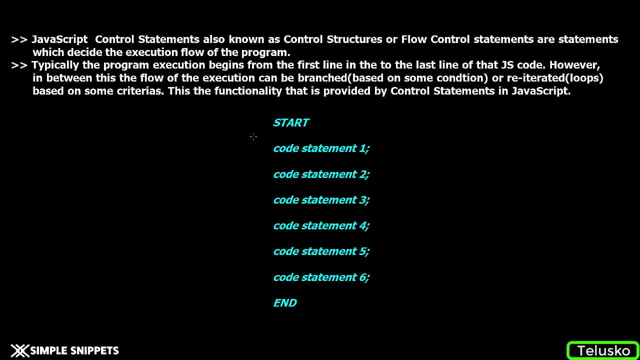 to be and how the code statements are going to be executed one after another. So why do we need these control statements? Now, let's say you have your program and you are running your program, So your JavaScript code is running. and let's say you're on line number three. 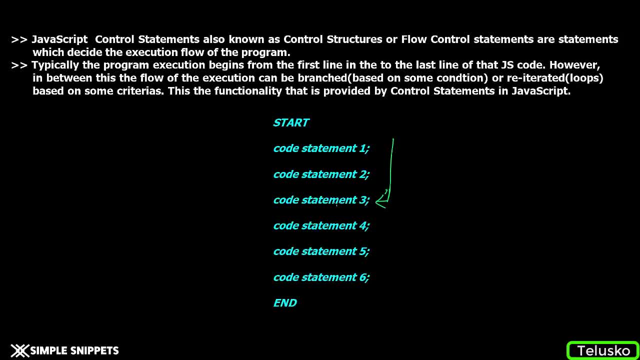 Okay, Your program has reached line number three, And now what is happening is you want to run this statement- that is, whatever instruction is there in this statement- a hundred times. Okay, Let's say you want to perform this one single statement, You have to perform a hundred. 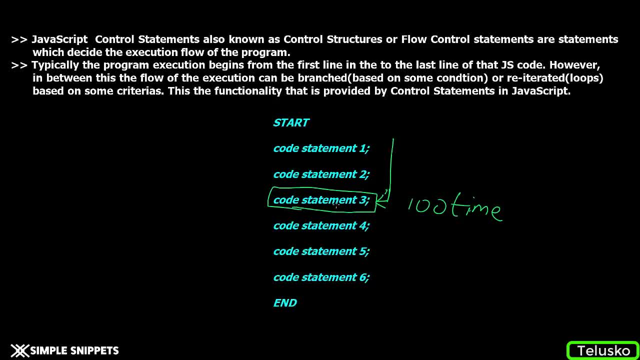 times? So in that case, are you going to copy paste this statement a hundred different times? No, right? It doesn't seem logical or it's totally useless, right? And it is unnecessary work, right? So what would you do in that case? So this is where that control statement. 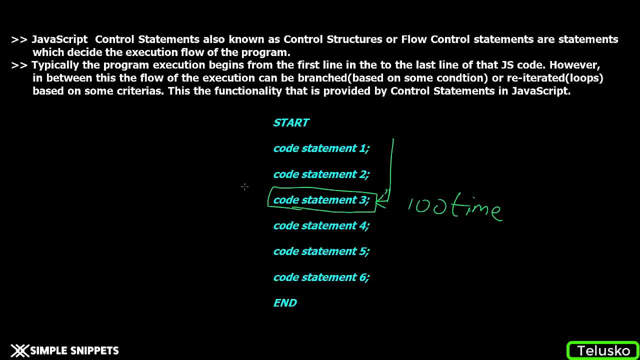 comes into picture and we'll talk about that in a minute. but let's take another case. So let's say, at line number five, you have to decide whether an integer is even or even Even number or an odd number. Okay, So let's say at this statement: you have a variable. 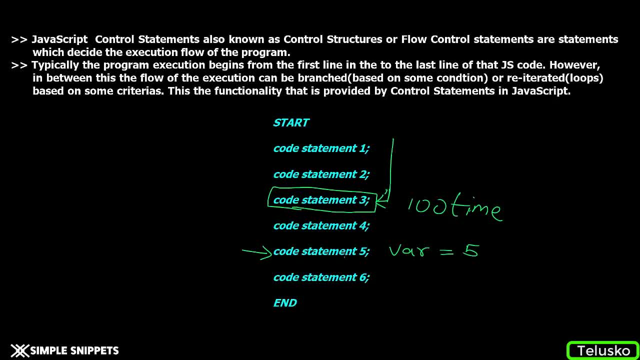 and you are storing some value over here. Let's say it is five and you have to make a decision whether this variable is an even number or an odd number, right? So in that case, two cases can happen: Either it is odd or it is even right. So this means that there. 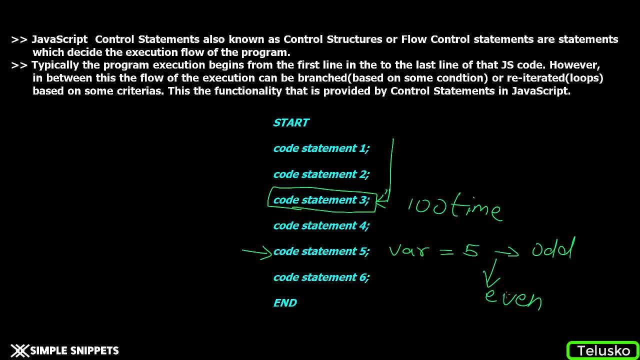 are two different branches and, depending upon what the result is, you can print or notify that it is an odd number or even number, right. So there are two different ways in which it can go. So this is where that branching is happening. So again, this is another example. 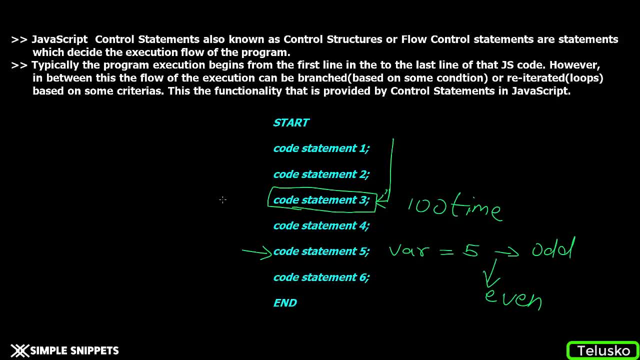 of control or control statements in JavaScript. So, in very basic terms, this is why we actually need control statements: so that we can perform certain activities and number of times or we can make certain decision making kind of scenarios wherein we can use these control statements. Now, in JavaScript, we basically have two different types of control statements.